0. And then we have x to be 1.. And then we have y to be 0. And then we have x to be 0. So we have x to be 1.. So we have x to be 1.. And then we have y to be 0. And then we have. 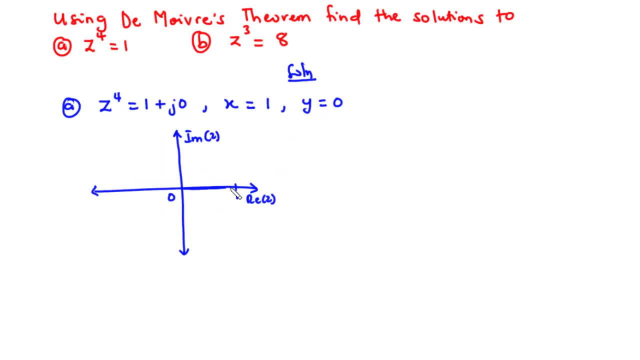 1 plus j0 is going to lie on the positive x-axis, So that is 1 plus j0.. So now let's find the value of r. So we know that r, which is the modulus, is given by the square root. 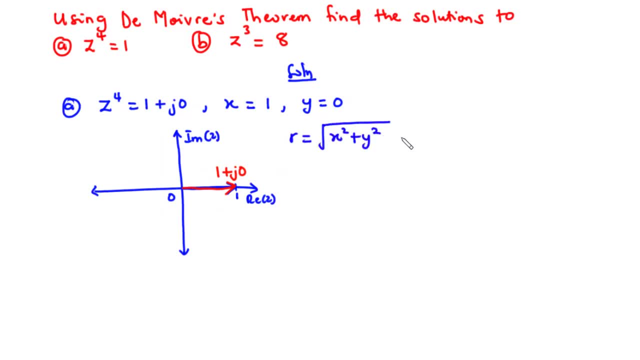 of the x component squared plus the y component squared, And that is equal to. we have the x component to be 1, so 1 squared. y component to be 0, 0 squared, And that is equal to the square root of 1.. Now the square root of 1 is equal. 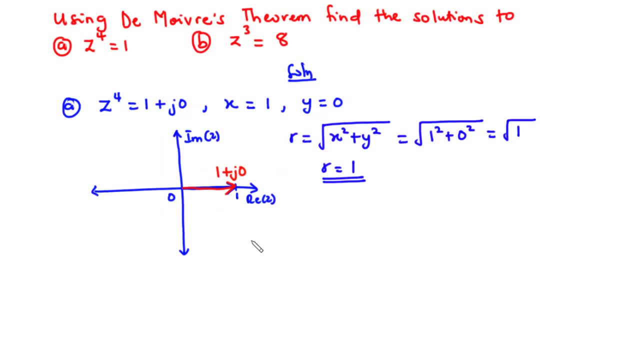 to 1.. Therefore we have the modulus to be 1.. Now let's find the value of the angle theta. Now, since 1 plus j0 lies on the positive x-axis, then it is evident that the angle between the complex number is 1.. So we have x to be 1.. And then we have y to be 1.. So that is. 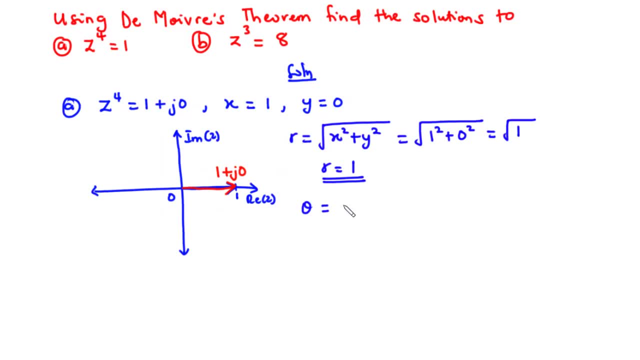 equal to 1.. So we have x to be 1.. Now let's find the value of the angle theta. Now, since 1 plus j0 lies on the positive x-axis, then it is evident that the angle between the complex number and the positive x-axis is 0. Therefore the complex number z exponent. 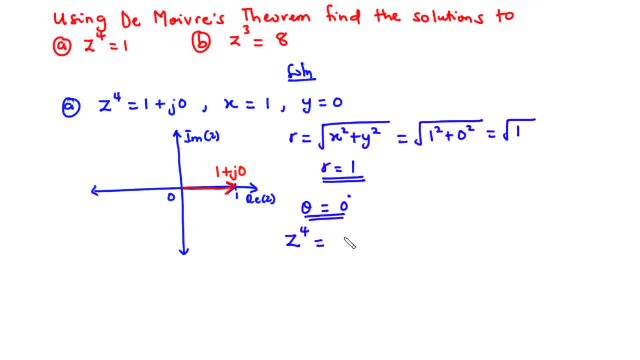 4, which is equal to 1 plus j0, can be represented in the polar form as 1 polar 0 degrees. Therefore, z exponent 4 is equal to 1 polar 0 degrees. Now let's make z the subject, So in doing so, we are going to multiply the exponent. 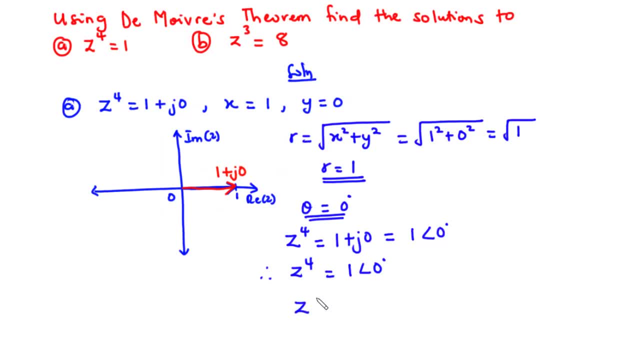 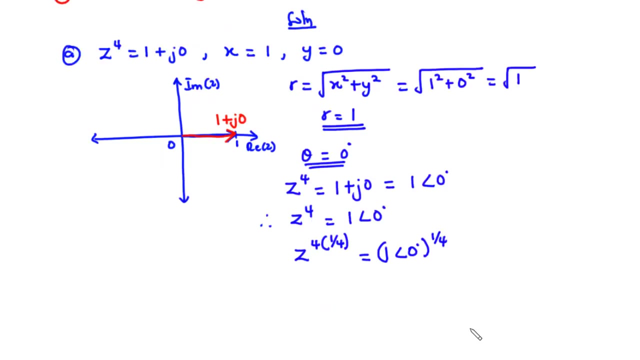 by 1 over 4.. So that becomes z exponent 4 times 1 over 4.. And then we do the same for the right-hand side. So we have 1 polar 0, all exponents 1 over 4. So that we have z. 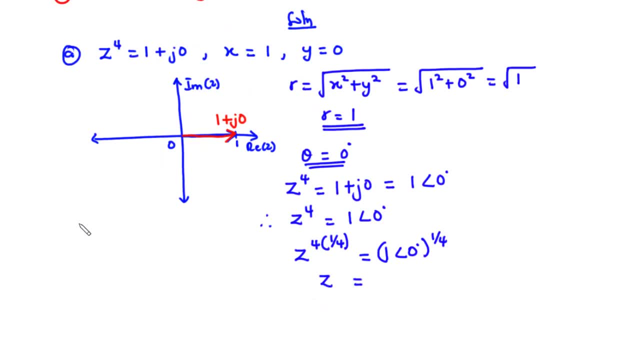 equals. Now, according to the Morbius theorem, we know that z exponent n is equal to r polar theta, all exponents n. So we can simplify that as r exponent n polar n times theta. So basically, that's what you are going to. 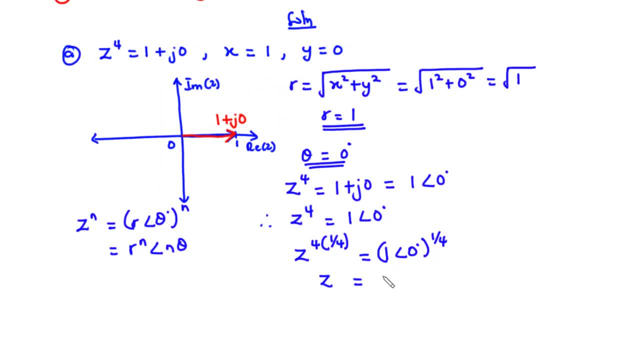 do here. So using the same theorem, we have 1 exponent 1 over 4 polar, 1 over 4 times 0 degrees, So that becomes z equals. Now 1 exponent 1 over 4 is still 1.. And then 1 over 4 times. 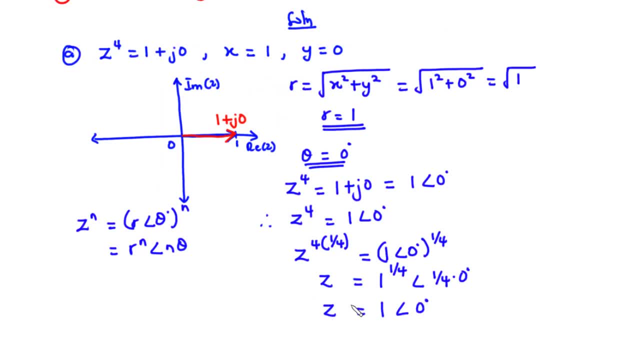 0 degrees is still 0 degrees. Therefore, this happens to be the first solution to z. exponent 4 equals 1 plus j0.. Now, since we have z to the power 4, it means that we need to arrive at 4 solutions, or 4 roots, And we have z1, which is the first solution. 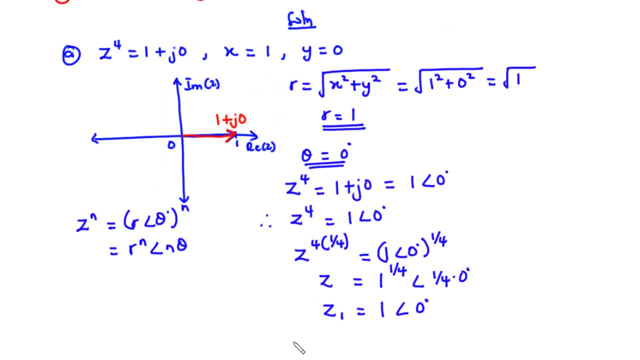 And we have z2, z3, and then z4. Now, how do we find z2, z3 and then z4?? Now, the roots of a complex number have the same modulus. The difference between them is they are symmetrically. 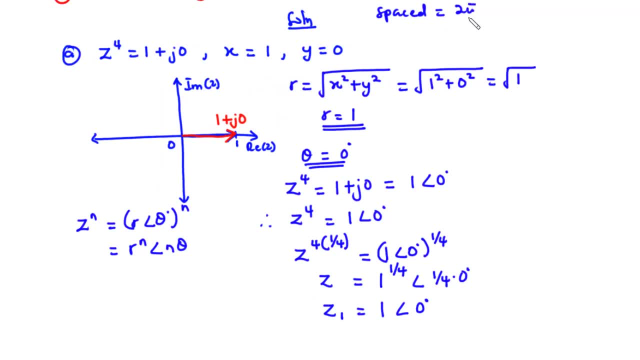 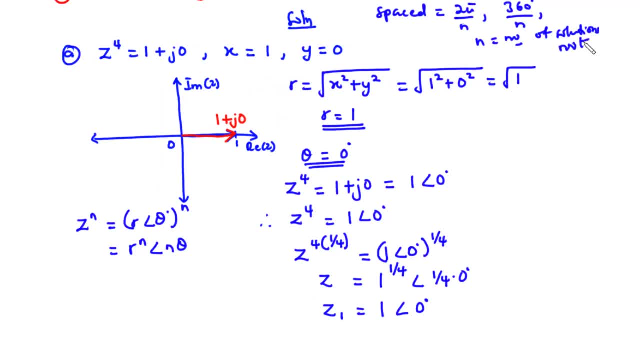 So the number of roots, So the number of roots, So the number of roots, number of solutions, or the number of roots. Now, since we have z to the power 4, which means that we have 4 solutions. therefore, we can say that the solutions to this complex number 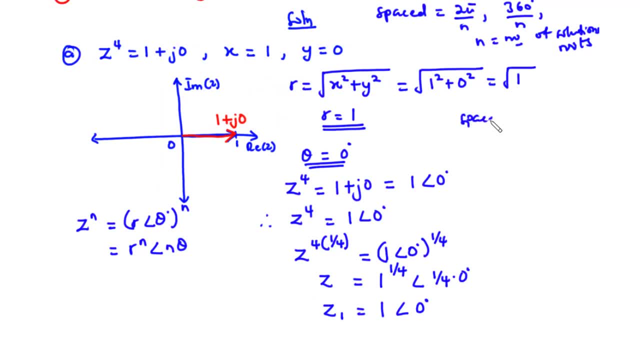 are symmetrically spaced by 360 degrees divided by 4, which is equal to 90 degrees. Therefore, if z1 is equal to 1 polar 0 degrees, then we have z2, to be equal to. the value of modulus remains the same, so we have 1 polar, and then we add 90 to this angle, so that we have 1. 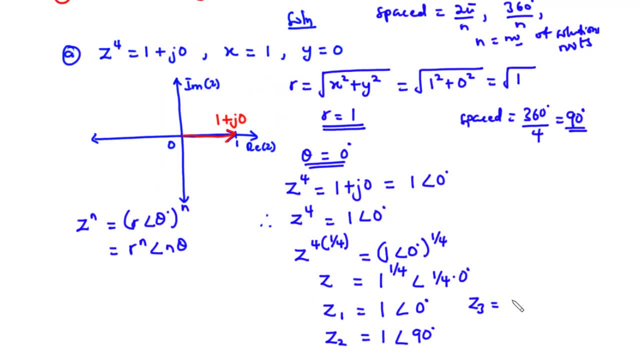 polar 90. also, for z3, we have 1 polar. we are going to add 90 to this value, that becomes 180.. And for z4, we are going to add 90 to 180, so that we have 270.. So therefore, these are the roots of the complex equation. z exponent 4 equals 1.. 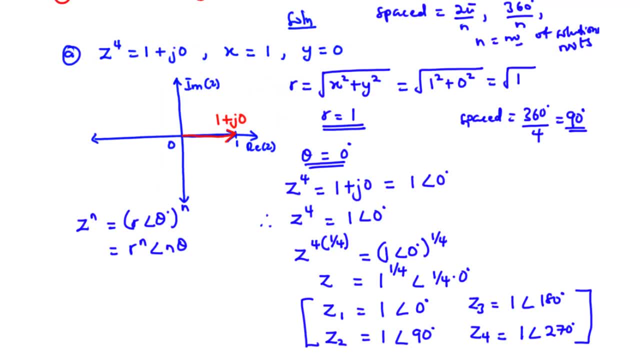 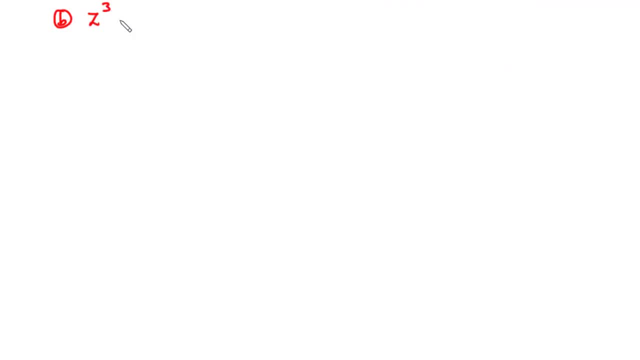 Now let's move on as we solve for b. So for b we have the complex equation: z exponent 3 equals 8.. Now we can express this as 8 plus j0, where we have the x value to be 8 and the y value. 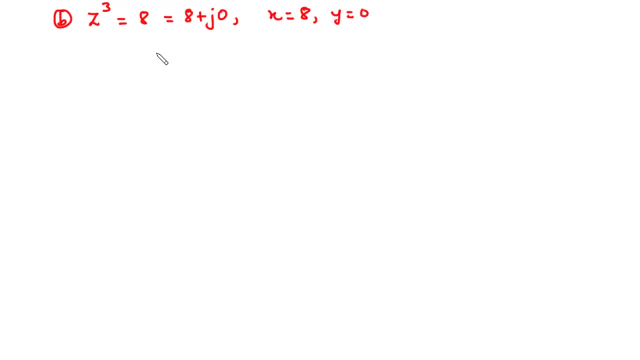 to be 0.. Now let's represent this on the Argand diagram. So we have the x value to be 8 and the y value to be 0, which means that we have the complex number going to lie on the positive x axis. 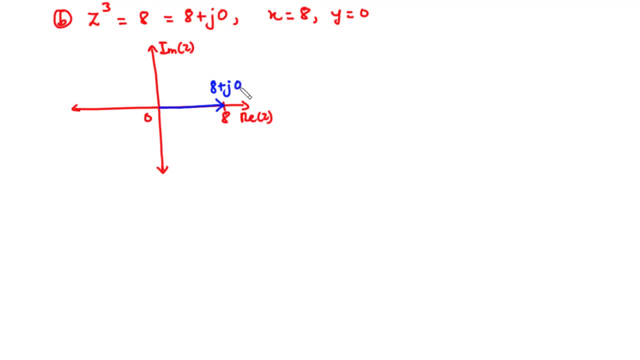 So that is 8 plus j0.. Now let's find the values of r and t. So we have: r equals the square root of x square plus y square. that is equal to 8 square plus 0 square. Now 8 square is 64.. 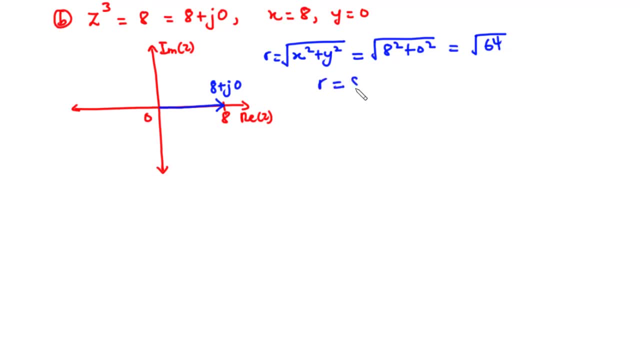 The square root of 64 is 8.. So we have: r equals 8.. Now, since the complex number lies on the positive x axis, The angle between r, or the complex number, and the positive x axis is 0.. Therefore z cube, which is equal to 8 plus j0, can be represented in the polar form as: 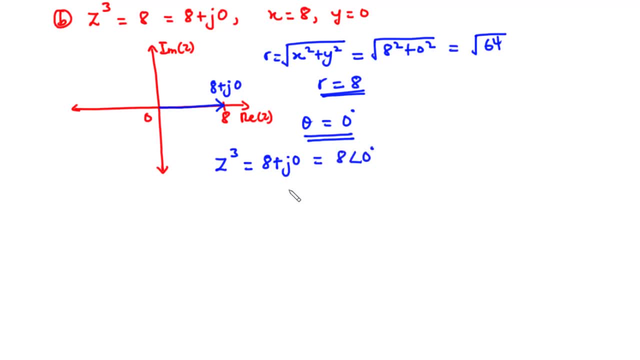 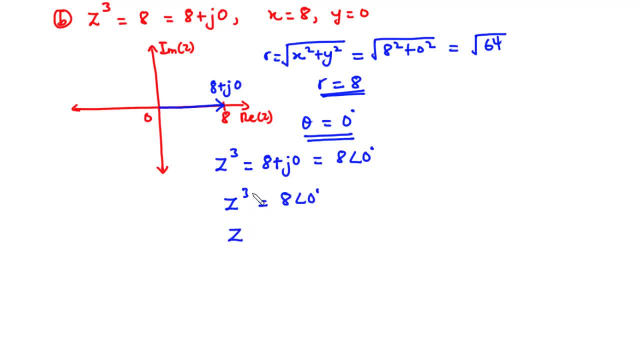 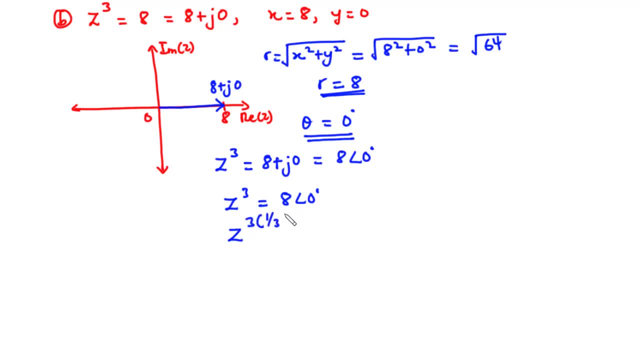 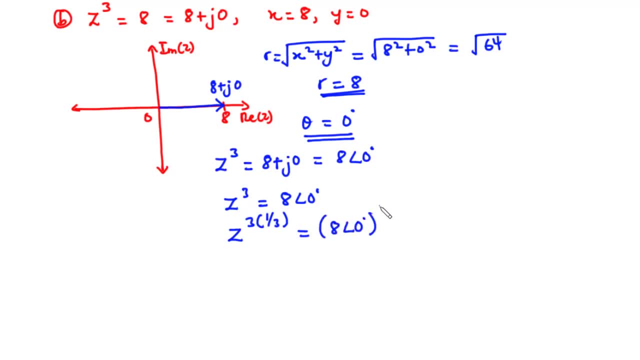 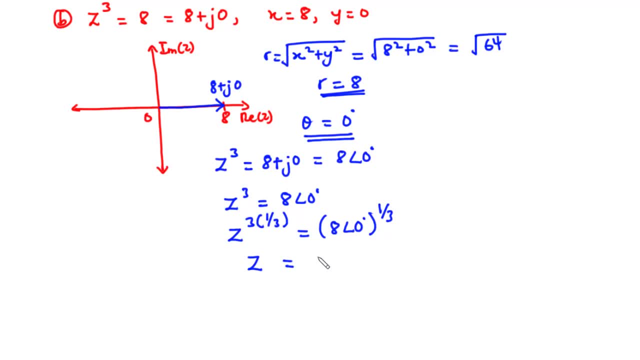 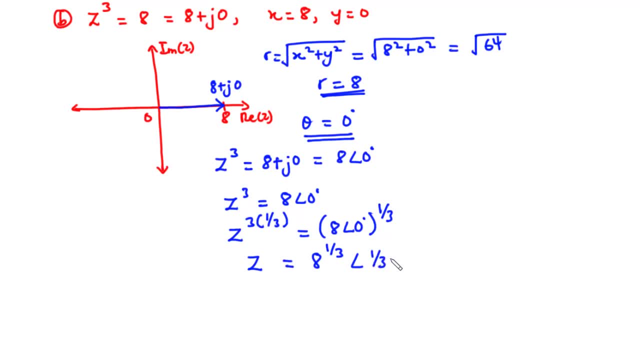 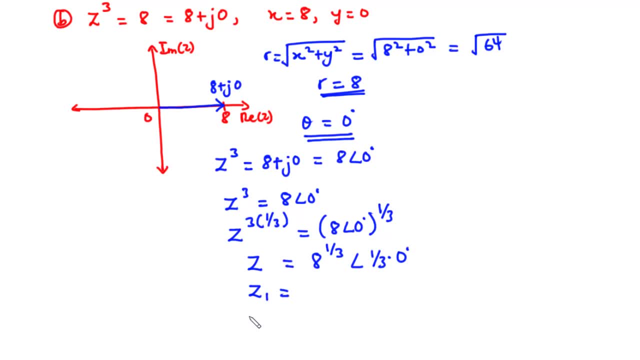 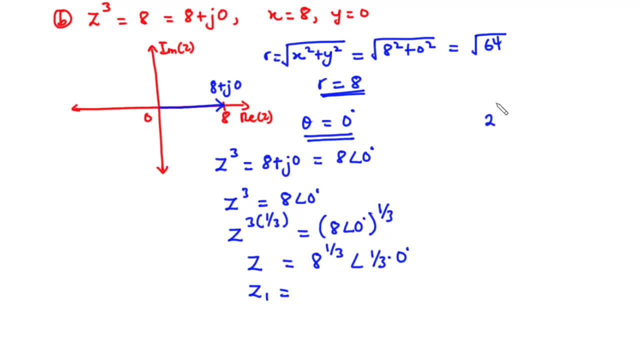 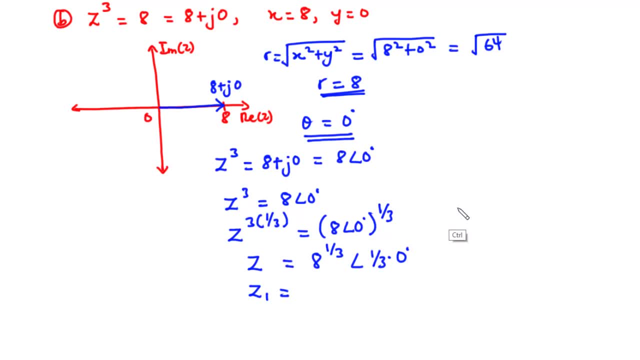 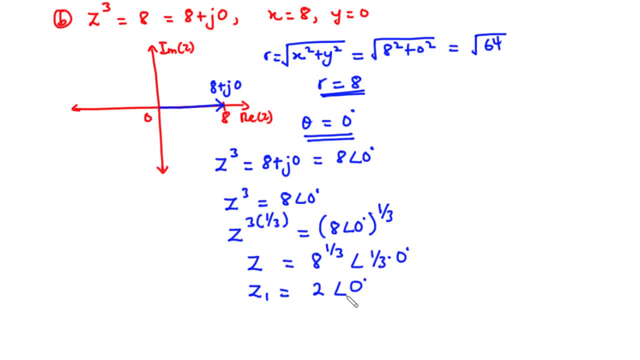 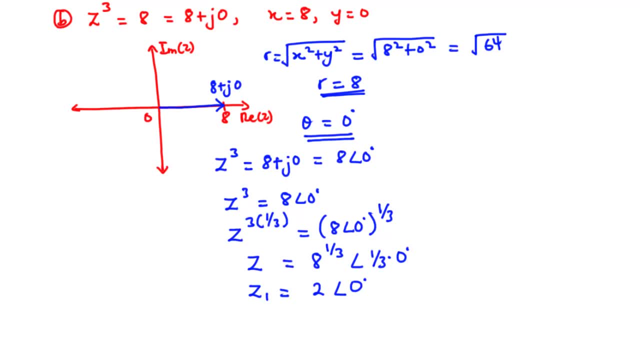 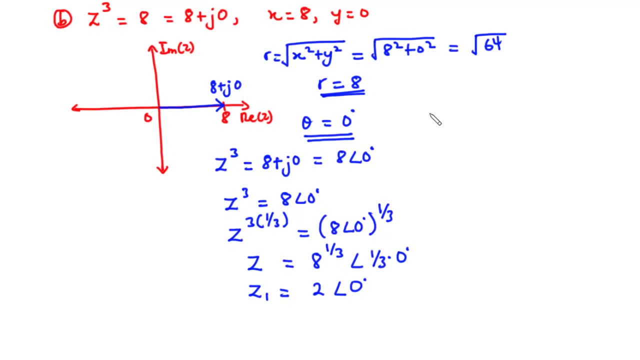 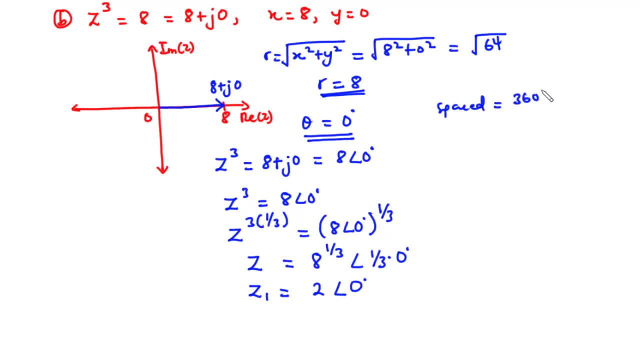 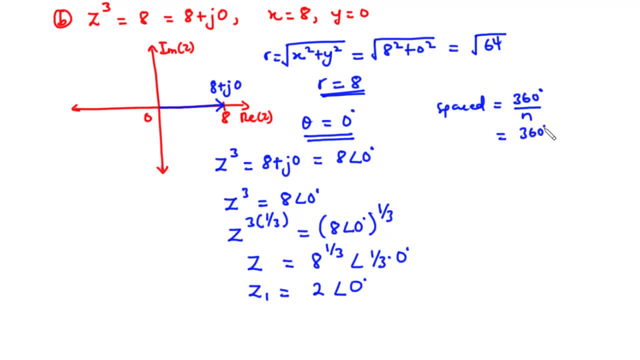